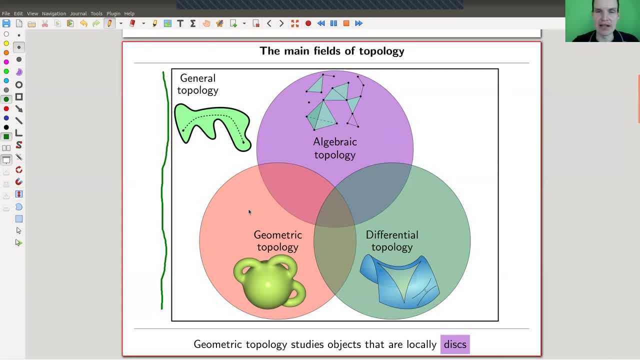 you can see it here- which is this general topology. that language underlined topology, but i said continuous functions and topological topological spaces. pass tikhanov's theorem, something like that, and then you have three main fields of topology, roughly speaking of course, and they are huge intersections. it's quite a venn diagram, as you. 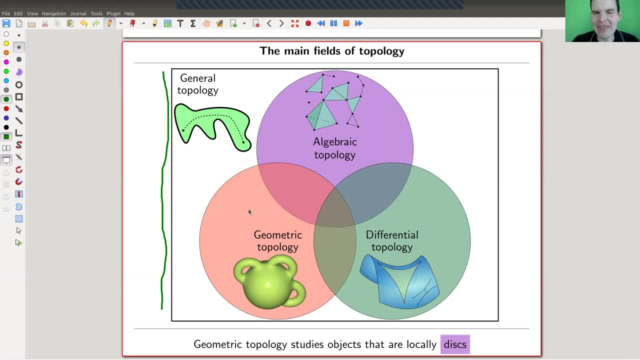 can see here. so you have algebraic topology, which is kind of the study of algebraic invariants associated to topology or topological object, which depends a bit how you want to interpret it. it's more part of algebra than topology itself, but okay anyway. so it's really about combinatorial objects like cw complexes or 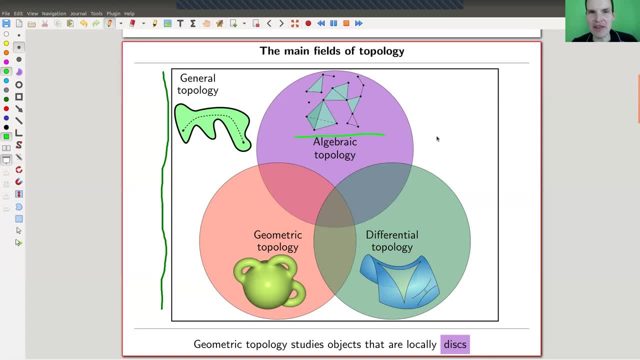 some cell complexes like like this stuff here. differential topology is what the name says. it's topology with some extra information. you might have a metric around or some differential structure, some smooth structure, something like that. and geometric topology is the geometric part of topology. topologie, just kidding, it's kind of the study. 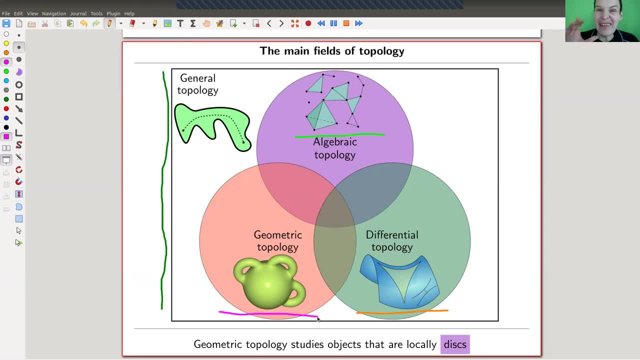 of many forms. that's what it is, and so the study of things that are locally disks. so these are called many floors. and here's an example of a manifold: severe, with three handles, kind of the easiest belt, certainly not the easiest non-trivial example. it's any example of a manifold. but let's actually get started and try to motivate where everything 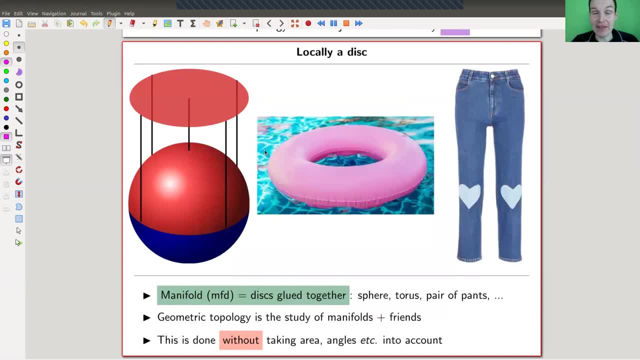 comes from. so really the study of geometric topology is not a geometric topology, is not studying random topological spaces. there's nothing butizzaging. you know we can buy cold. There's not really much you can say about general topological spaces. That's something you should do in general topology anyway. 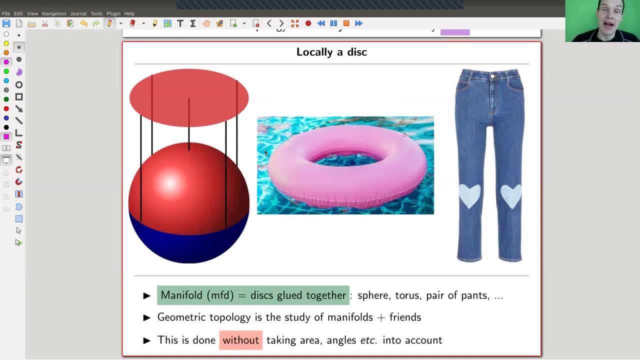 So we're doing geometric topology and geometric topology a very, very applicable field, by the way. So geometric topology is a study of manifolds. So I shorten that, of course, because it's way too long as a word, It's a mouthful, And the manifold, basically speaking, roughly speaking, is just something that is glued together from disks. 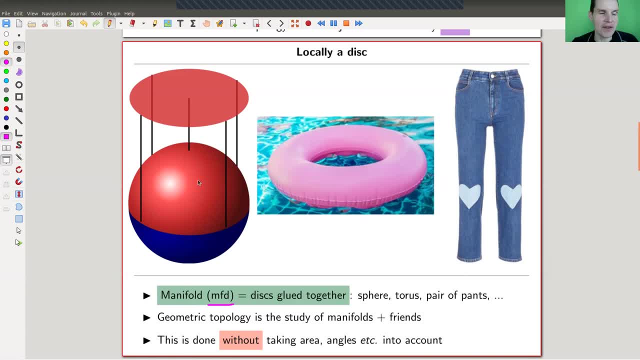 So, if you think of something like a sphere of the northern hemisphere, of the southern hemisphere and basically the northern hemisphere, if you ignore the rest, here is just a disk, as you can see. Well, maybe not, because I've chosen a bad color here. So, as you can see, this is just a disk. 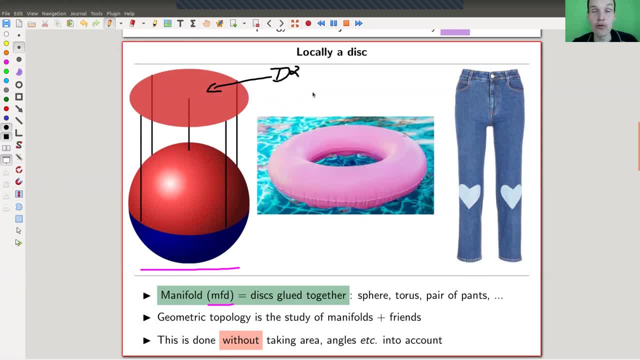 So this is a d2.. d is a disk and 2 is the dimension of the disk. So d2.. Same for the southern hemisphere. You can find smaller disks here and you can glue them together. Yes, Again, quite a Venn diagram here. And there's another disk. 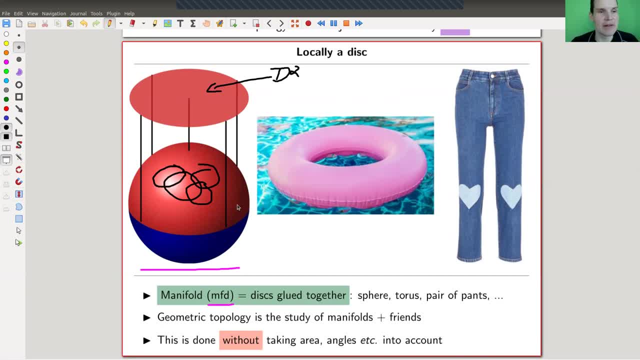 So this space is certainly locally made out of disks, But so is this space, which I will show you, a nice Mathematica code that you can run yourself. Well, it's not code, it's a demonstration that you can run yourself, linked in the description. 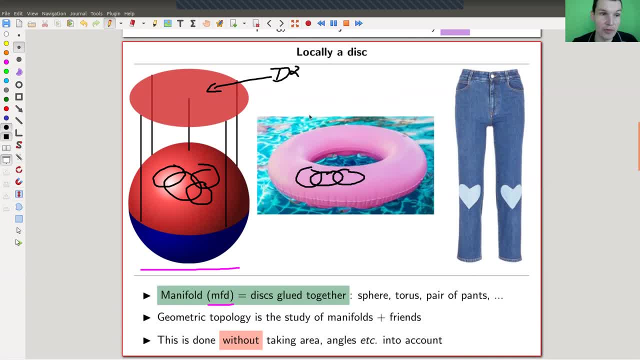 So this swim ring type object, sometimes called a torus, is also locally made out of disks And you actually really can't tell locally. that's the whole point. Locally you can't tell whether this is a flat disk or not. 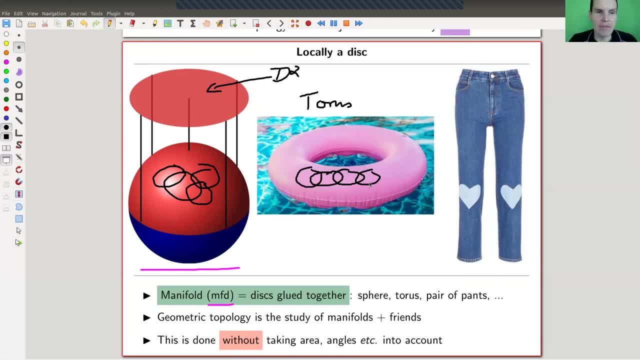 We'll see that in a second. Just here as a slight remark. So the torus is not a donut. A lot of people say the torus is a donut because the torus is really more of a swim ring. It's hollow inside. 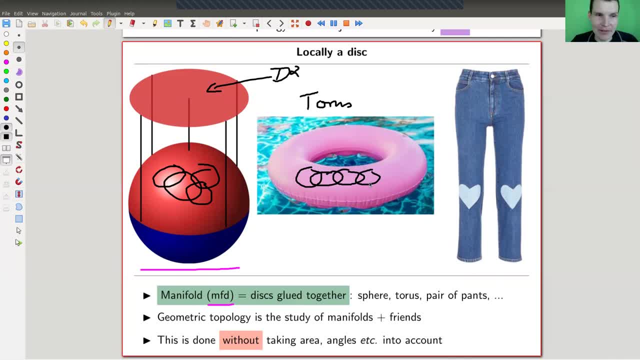 I don't know what kind of donuts you like, but a hollow donut would be a little bit disappointing, I guess. Anyway, so people usually call it a donut. It's more like a swim ring type of object. Keep that in mind. It's really, really hollow. 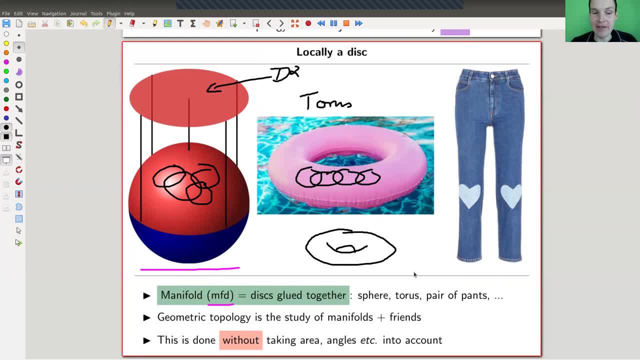 So there's air inside, if you want. Another example of a manifold is your pair of pens. I hope you're wearing a pair of pens right now. If not, well fine, It's fine with me, But anyway. so if you're wearing a pair of pens right now, that's a manifold. 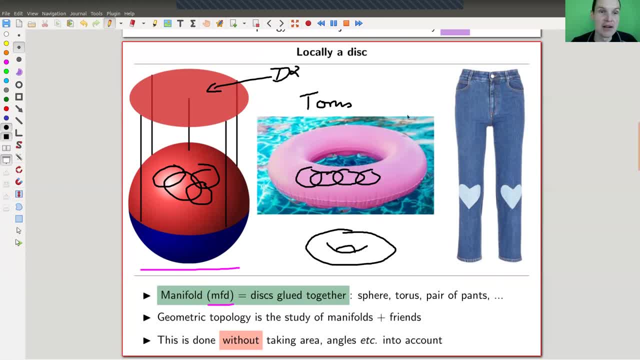 And how can you check that that's a manifold? Well, if you ever had a patch on your pair of pens, that's your local disk. So again, you have lots of local disks here on your pair of pens. So it's a manifold. 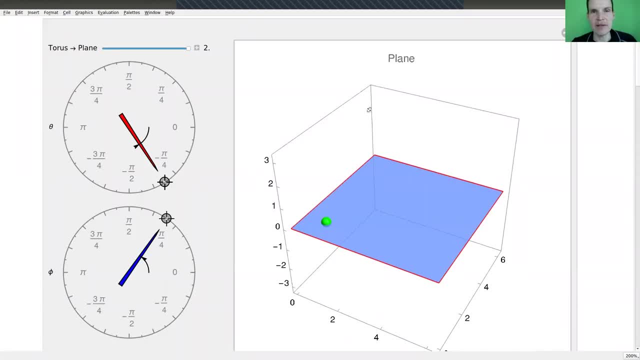 So let's zoom into the torus. So here's a nice mathematical demonstration which is, as I said, linked in the description. So the torus is a two-dimensional object. Keep in mind: it's hollow, So it's only the surface area of the torus. 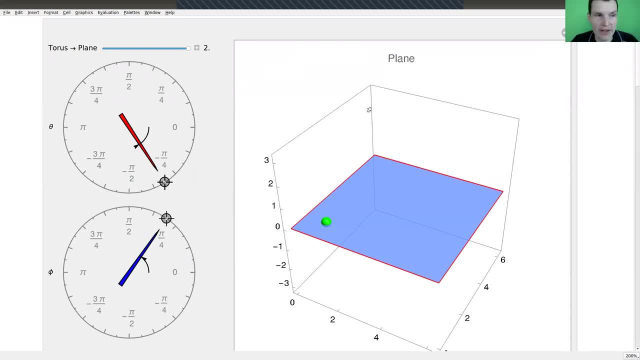 And you can parameterize it by using two coordinates And you can kind of play around here with those coordinates and remove the greenish dot here. So we have two coordinates which are given in polar coordinates, So two angles basically, And what you can do here. 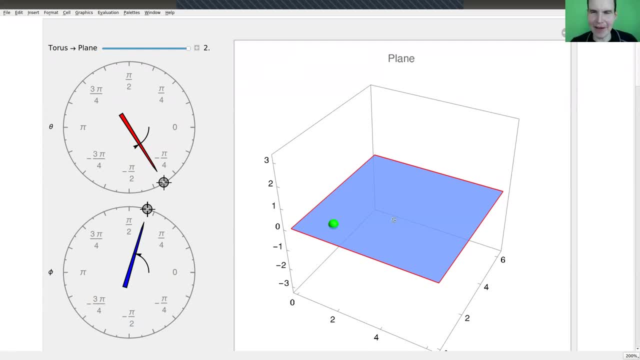 So this you might want to complain. now This doesn't look like a torus- Neither like a torus nor like a donut, nor like a swim ring. The point is, this is a local picture. You should really think that you are this green little ball or whatever it is. 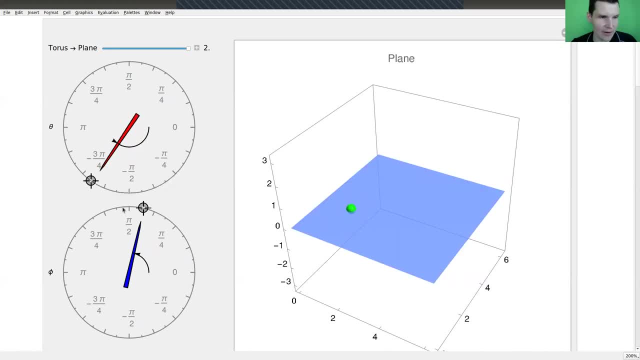 And you really can't tell whether you're locally on a disk or whether it's a torus. It is a torus. So let me show you that this is not just a rectangle. So if you move out here, it actually ticks back. 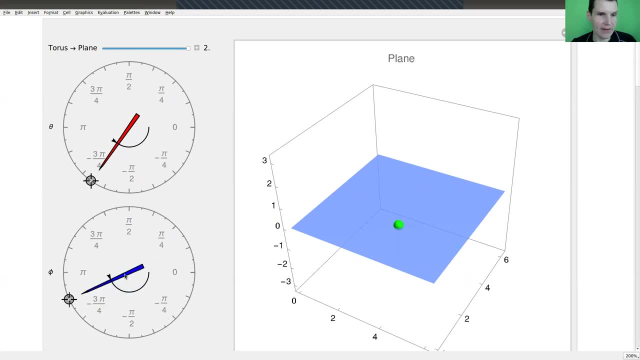 And comes back And comes back in from the other side, Which is on the rectangle, a non-continuous movement, But on the torus it's completely continuous And same. here It ticks over And comes in on the other side. 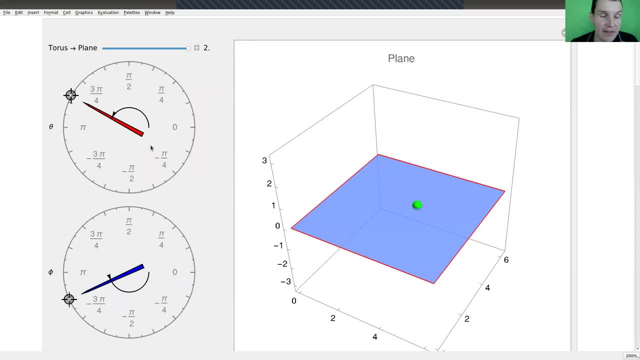 But locally you simply can't tell whether it's a disk or not, And that's the whole point. So let me construct now the torus for you, So you can actually pull this little bar. And what it does is: it then constructs the torus by identifying the sides of the 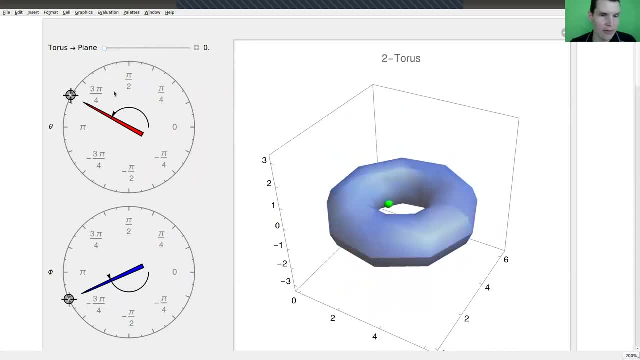 Of the rectangle And this is then the torus. So here you go, That's a swim ring, And you can do the same movement on the swim ring And it's really just the same movement. It's just locally explained, or not locally. 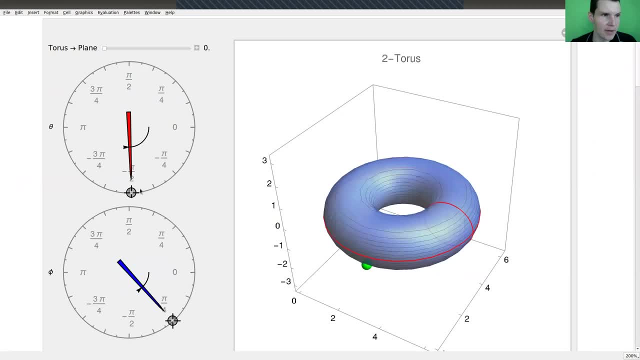 So this one, the one that was kind of going around, is jumping around on the rectangle. If you left it to one side, you come in to the other side. It's really just this operation: that you go around the torus Or you go around the hole. 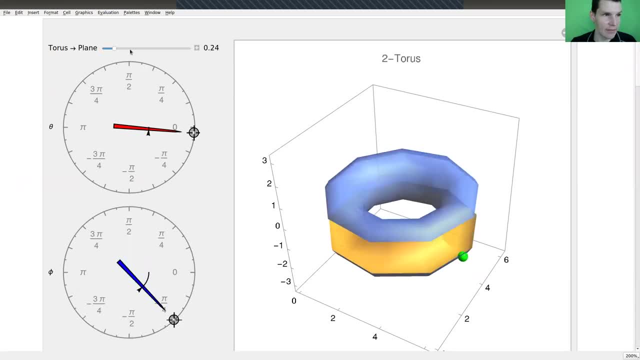 And that's basically it. So this is the two directions. And then if you flatten it out again locally, you really can't tell the difference. It's whatever it is. You really have no idea, you can't tell the difference, And that's a manifold. 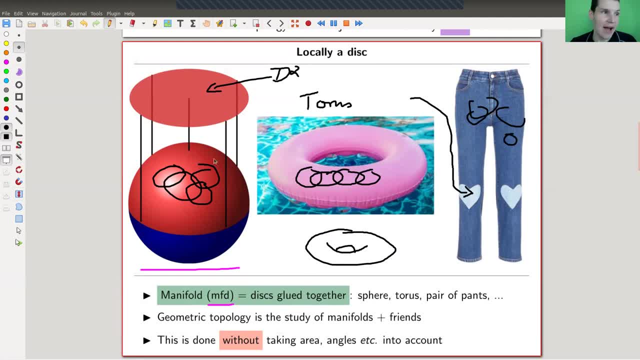 But so locally we can't tell the difference from a disk, And by a disk I really in the end mean a, d to the n, So there might be an n-dimensional manifold. It's just a bit harder to imagine. So two dimensions is really really good for our brains, at least for my brain. 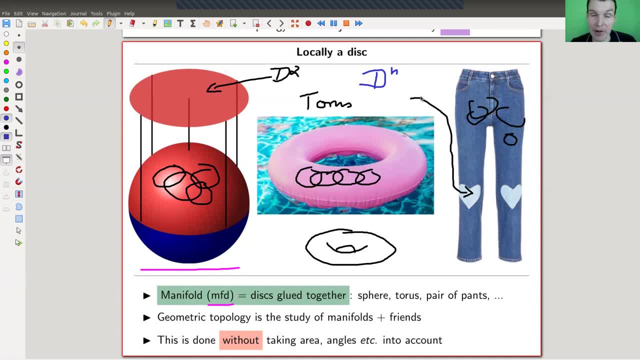 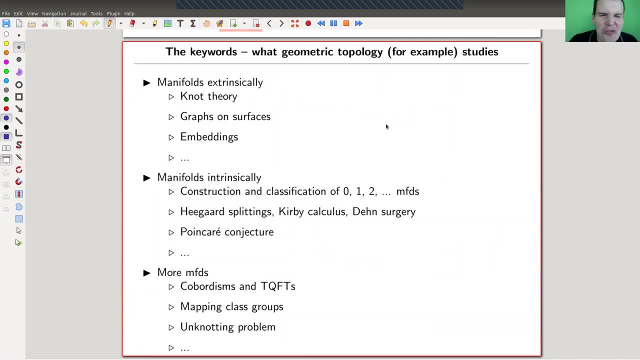 So I stick here On the slide with two dimensions, But eventually we'll see higher dimensional spaces. So it's kind of the outline of a classical course on geometric topology, whatever that means. And basically what I'm trying to cover is extrinsic properties of manifolds, which really means you just kind of fix something additional like an embedding. 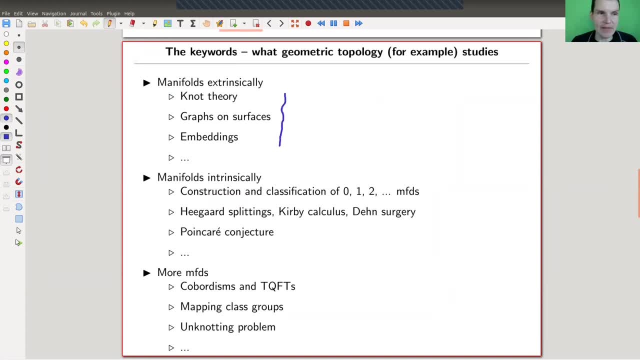 So I'm going to explain knots and graphs and embeddings, basically Kind of a lot of fun to begin with, And then the manifold's interface. So the manifold's intrinsically, which was really my little torus picture, was a green ball. 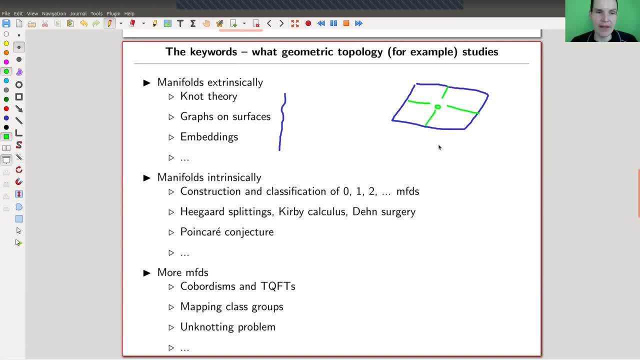 It was moving around the torus. That's really intrinsically. I can't tell whether it's a flat space or not as soon as I stand on it, And I need some idea how to tell that it's not a flat space. 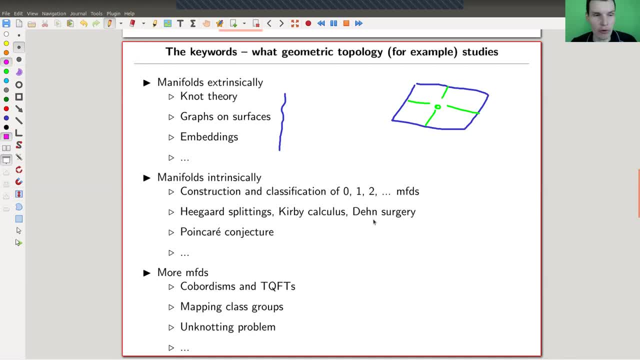 And this usually has some really, really kind of sophisticated topics. Somehow it depends a little bit on your dimension. So, construction, classification of mostly low dimensional manifolds, So I hope to get up to three and four Beyond that. it's just too crazy for me. 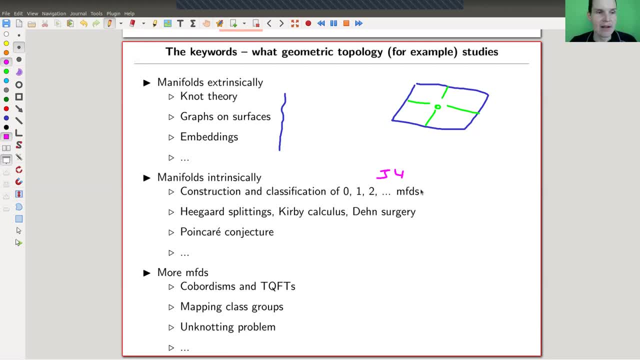 Probably three and four are already too crazy for me, But we'll see. In particular, in dimension three and four there are Heegaard splitting, Scurvy, calculus and certain types of Dehn surgeries, Dehn twists and so on. 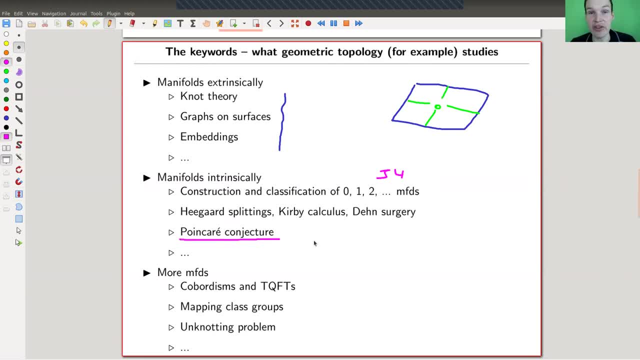 They're very important. And then there is the famous Poincare conjecture, which I will recall in a second, which I hope to cover somehow, Somehow, explaining even the proof, The statement or the status of the conjecture in four dimensions. 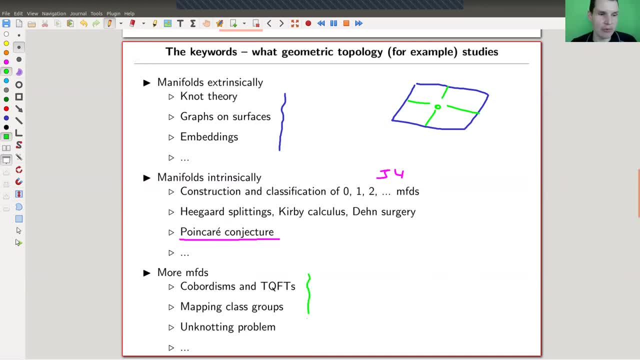 We'll see, And along the way we will have some other problems that are related to geometric topology. So you can think of maps between manifolds. That's usually also studied in geometric topology. So cobordisms, if you know what that means. 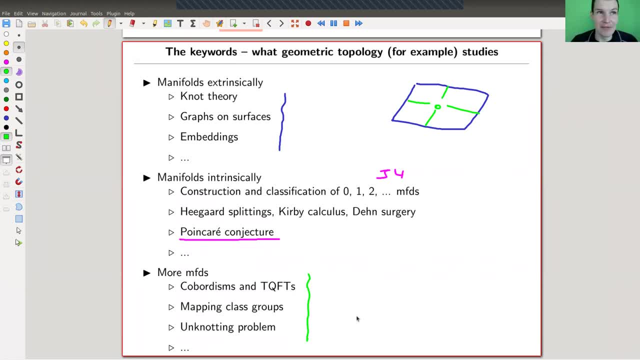 If not, we'll see what these are: Mapping class groups, That's just maps between the manifolds. And there are other problems related, like the unknotting problem, which is more A problem of complexity theory than of geometric topology itself. 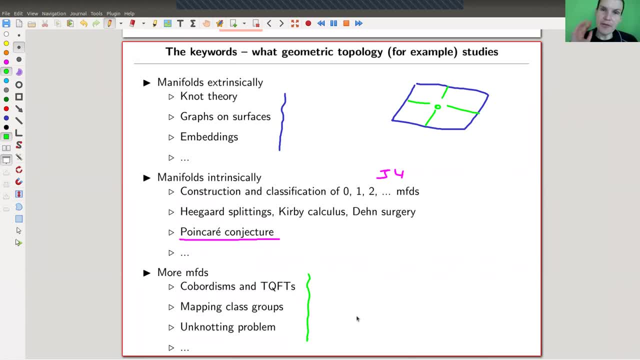 But we'll see. So kind of the outline is some funny knot theory which is a lot of fun, which is then manifold extrinsically. Graphs, manifolds extrinsically. A graph is not really a manifold, but I would put it on manifolds or something. 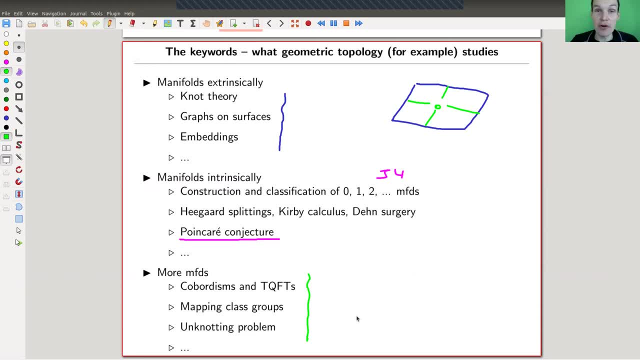 You will see embeddings. You can ask the question: what is the smallest space the torus lives in? Can it live in a two space? Can it live in R2?? No, it can't. Can it live in R3?? Well, let's have a look. 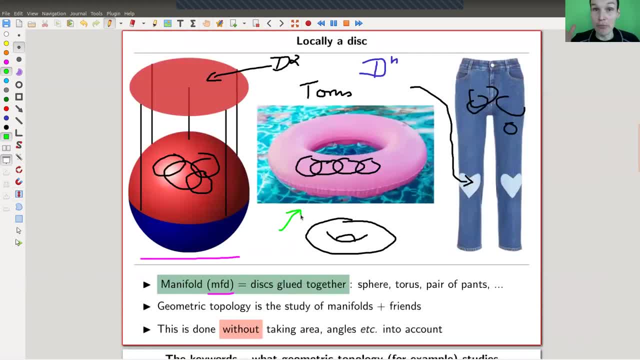 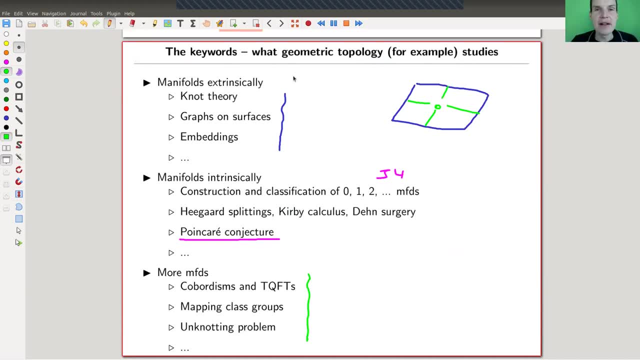 There you go It. can We have a swing ring Proof that it can live in R3. And so on. You can ask those questions for the minimal embedding or the minimal immersion, Something like that, Or, more intrinsically, stuff like Heegaard splitting. 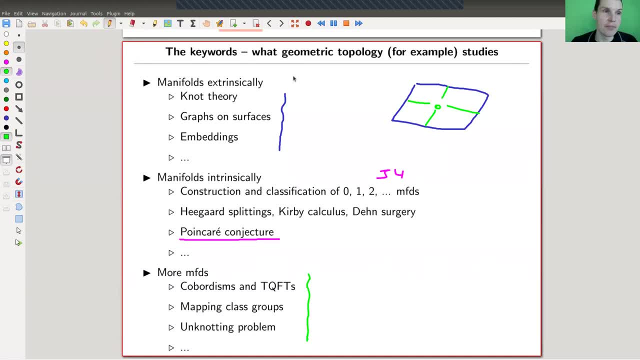 So Kirby calculus to construct manifolds in the Poincare conjecture. So not to construct a Poincare conjecture, So to construct manifolds, comma, in the Poincare conjecture. to discuss the Poincare conjecture. 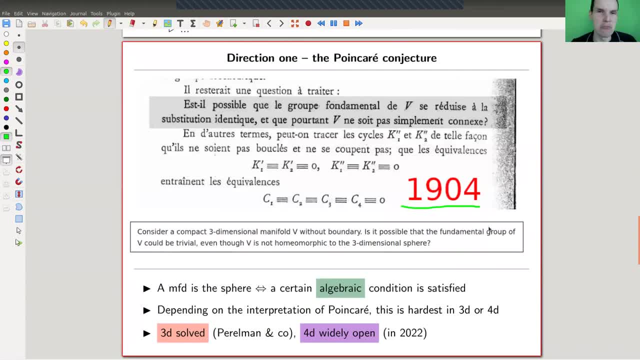 So the Poincare conjecture? The Poincare conjecture goes back to roughly well, roughly 120 years. by now, Let's say, 120 years doesn't matter so much, And it's a question asked by Poincare. 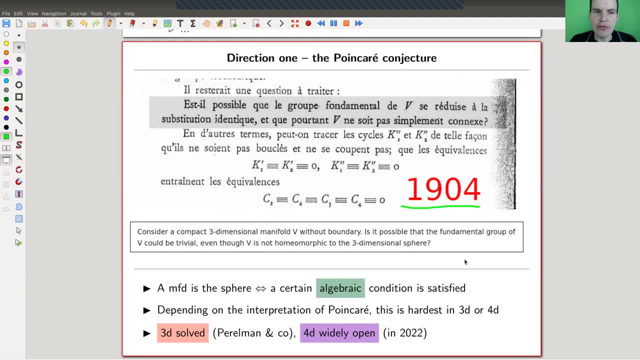 Basically, it's the following: So how much information do you need to detect whether you have a sphere or not, And in this case something like the three sphere. And basically the question was this: How much algebraic conditions do you need to determine whether it's a sphere? 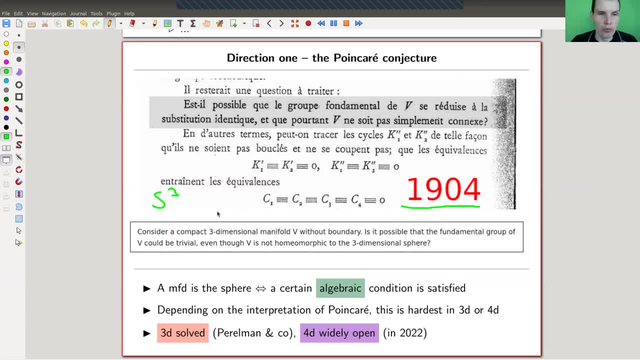 And that problem was widely open for a long time And roughly in the 80s, 90s, probably 80s- people developed tools to kind of try to address this Poincare conjecture which turns out to be hardest. 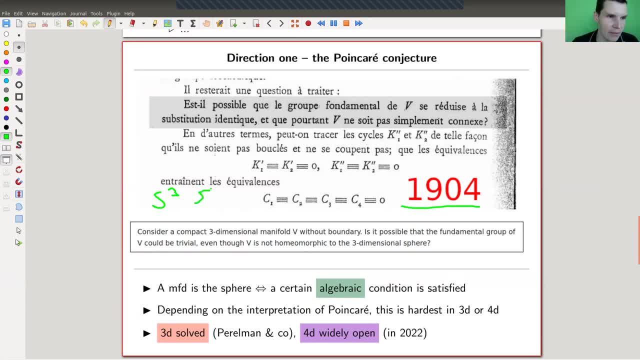 You can interpret this in any dimension, So you can do SN, for example, And it turns out to be hardest in dimension three. So in dimension three it's actually the hardest part. The hardest part of the conjecture is dimension three. 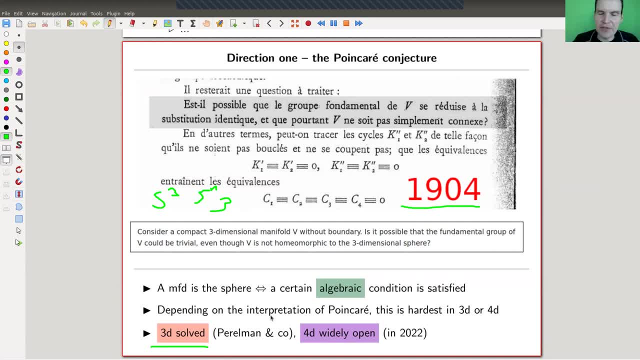 The rest was already known kind of in the 60s. So, as I tried to say, in the 80s people developed techniques to attack dimension three And it took about 20 more years until, very famously, Perelman then kind of solved it in three archive papers which were never published. 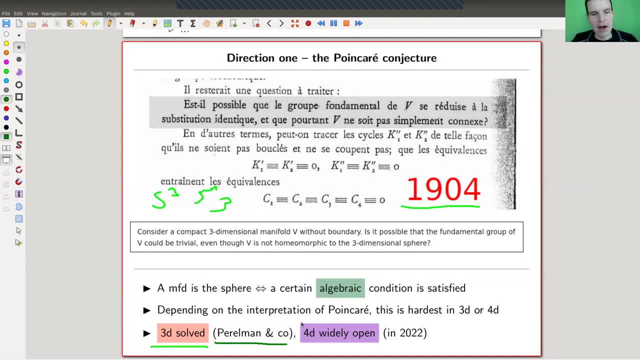 But basically the ideas were there And then people polished it. That sounds a bit unfair. It's still non-trivial to polish it, But basically people have polished it And nowadays it's known. It's the Poincare conjecture. 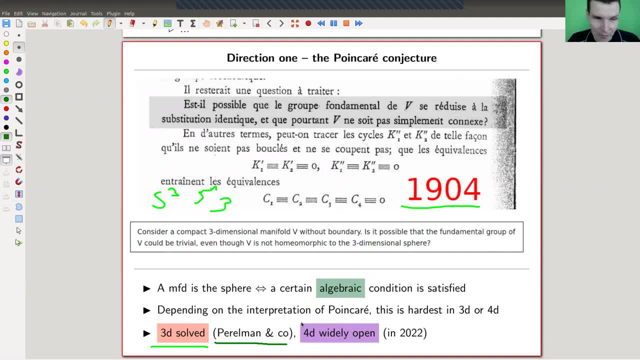 It's now a theorem, Whatever you want to call it, the Perelman and Go theorem, If you want. But then there's a funny part of topology. So, as I said here, in this 3D case, people from the 80s started to develop tools to prove the conjecture. 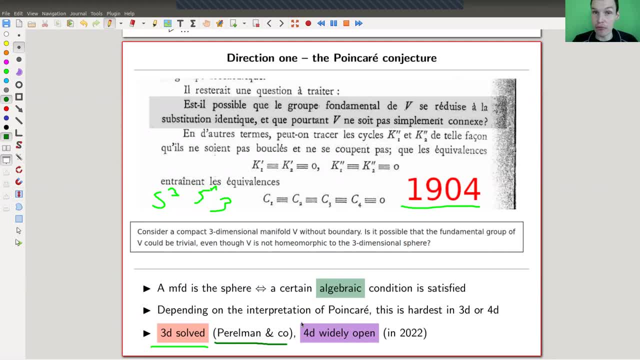 So it was kind of the experts that agreed that the conjecture is true. A conjecture doesn't need to be true, right, And depending a little bit how you interpret Poincare. So Poincare is not known to be, or certainly one of the pioneers of geometric topology, but also certainly not well known to be, super precise. 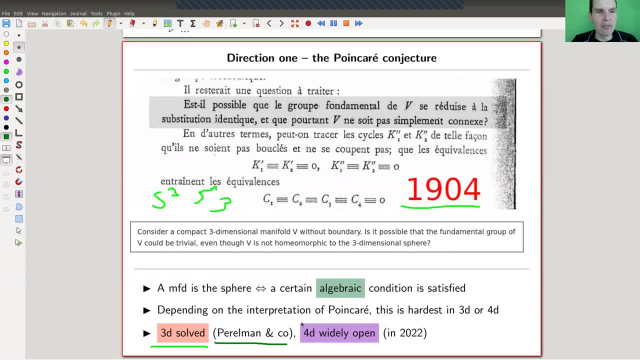 So Poincare is known by whatever is written in their papers. And well, it turns out that you can interpret Poincare's question about how can I detect spheres topologically like just as a topological sphere, or smoothly like as a smooth sphere. 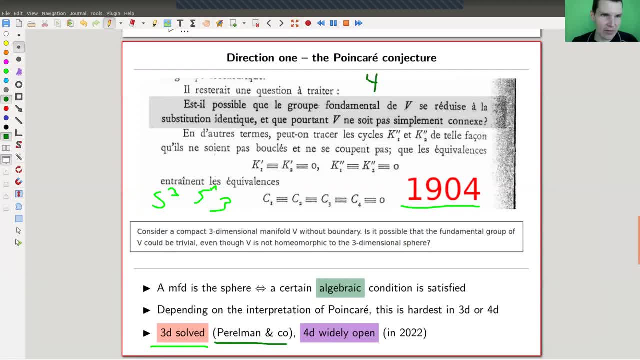 And it turns out that, smoothly, dimension 4 is actually the most complicated, not dimension 3.. The other dimensions are reasonably easy. And then you have the corresponding conjecture: How much algebraic information do we need? How much information do we need to detect a smooth sphere in four dimensions? basically, 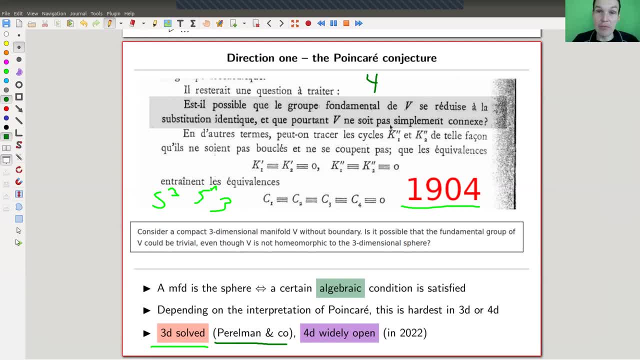 And well, in contrast to the three-dimensional one, which was famously solved by Poincare's conjecture, by Perelman, the 4D case is still widely open. And it's really really widely open in the sense that the experts don't even really agree whether it's true or false. 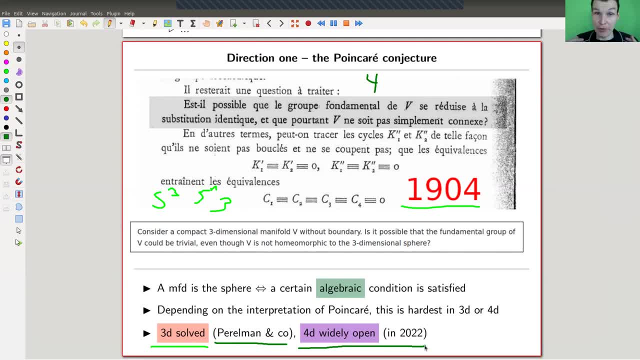 So there are certain people who try to disprove the conjecture. There are certain people who try to prove the conjecture And it's quite a mess. So I probably think I have no idea. It could be solved tomorrow. I have actually no idea. 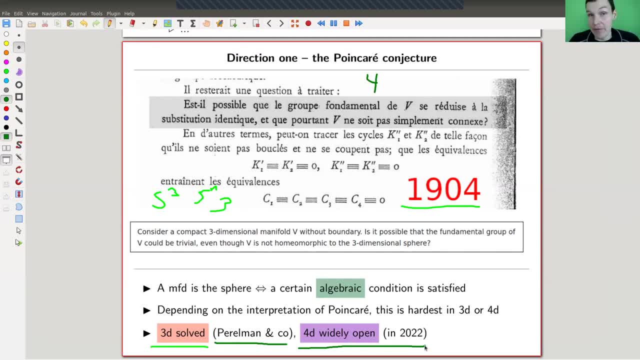 But I would guess that it will take a while to be settled, if it's ever settled. So it's really really hard. So it turns out that in this sense, low-dimensional topology- at least for this question- dimension 3 and 4 are the hardest, for some reasons I'm trying to cover in this video series. 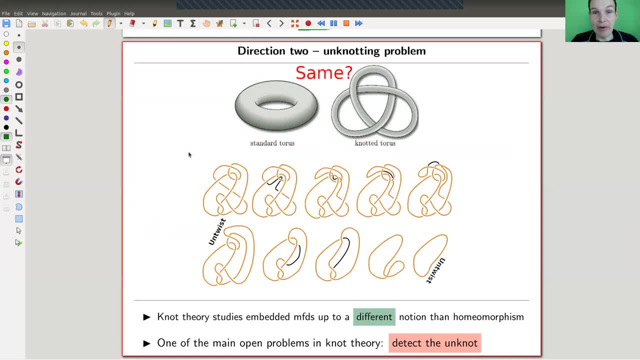 Anyway. so the unlocking problem is something very different in nature. So one problem you face with kind of the standard definition in topology. So people always try to tell you that the torus is the same as a coffee cup. Fine, that's true up to the correct notion of isomorphism, of equivalence. 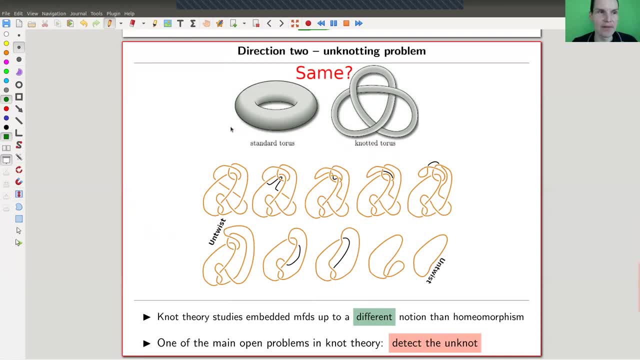 But that might not be the correct notion for what you have in mind. So what is here called the homeomorphism? So that's usually what you study intrinsically in manifold theory And would identify the homomorphism, The standard torus versus not a torus. 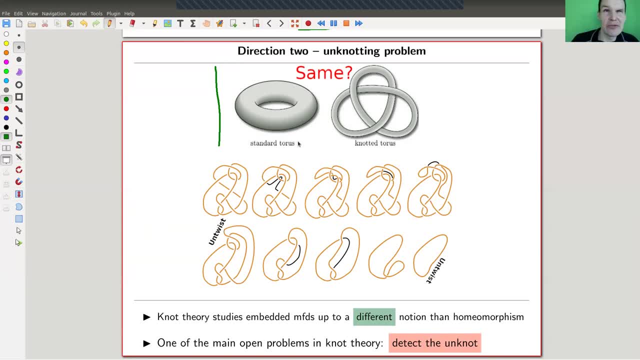 So if you want to do any kind of knot theory, a homomorphism can't be- at least not naively can't be- the correct notion And you come up with different notions of equivalence. You kind of take the embedding into account and see what that means. 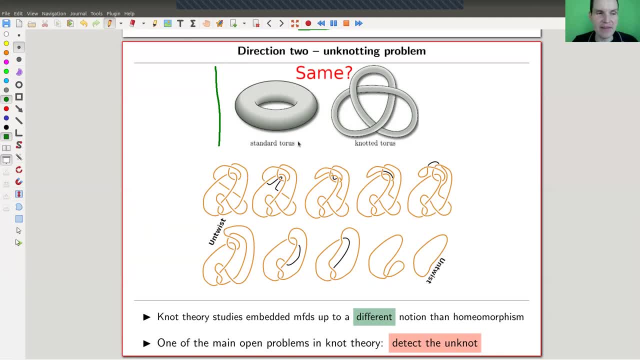 And then the question is: how can you detect knottedness basically? For example, here is a really really strange embedding of the unknot. It's just a circle. In the end you can undo this picture. It's quite trivial. 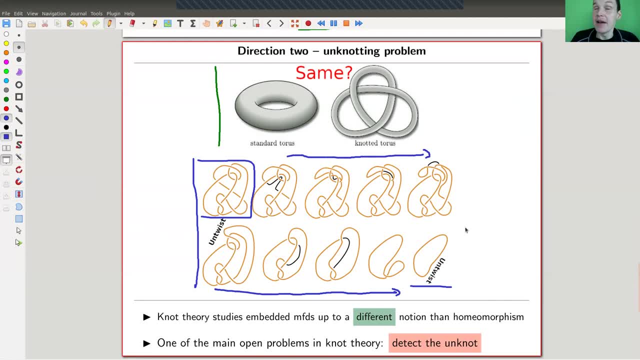 If you read along like here and you want to pause the video, I marked all the steps. It's not really trivial And to kind of answer the question, how hard it is to decide whether some mess, that you see some cabling of your computer cables or whatever, is really the unknot. 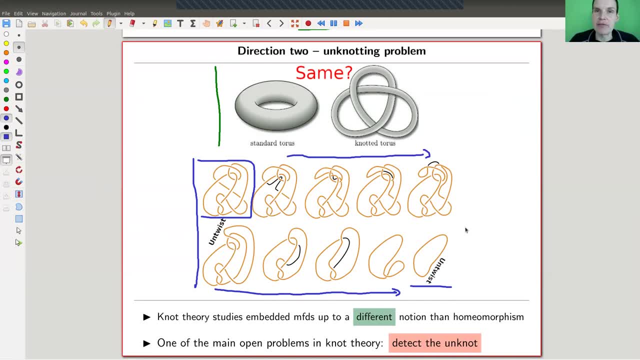 It's called the unknotting problem, which actually has some very nice connections to complexity theory and so on, And I also hope to cover this in this video series. Anyway, So geometric topology basically is the study of many folds in what incarnation ever. So in knot theory it's more like the embedding of many folds. And knot theory is not necessarily restricted to a circle in free space, It's just the easiest dimension. You can also think of a knotted surface in force space or something. 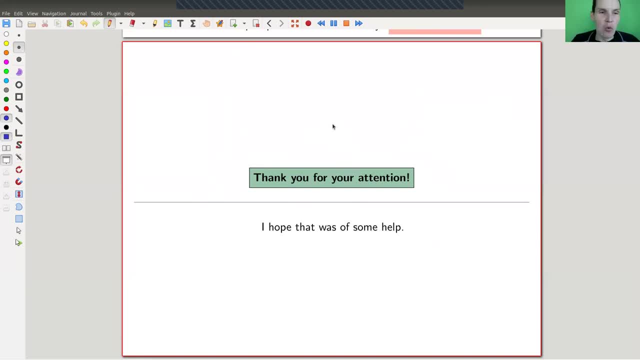 So knot theory is basically about embeddings, while kind of the rest of geometric topology- whatever that means- actually is also about intrinsic properties. How can you detect many folds, How can you construct many folds, Can you classify many folds? Poincare type conjectures, which is basically trying to find a good algebraic notion, how to detect the sphere, which is the easiest non-trivial manifold, and so on.